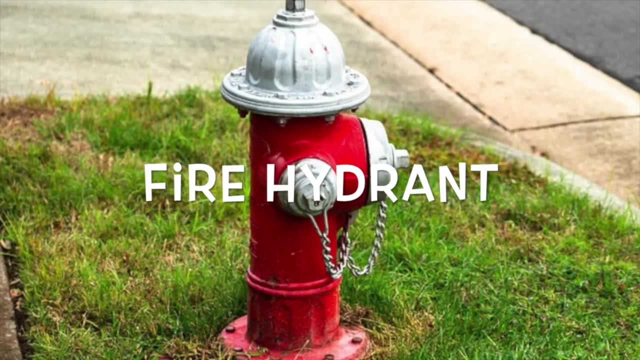 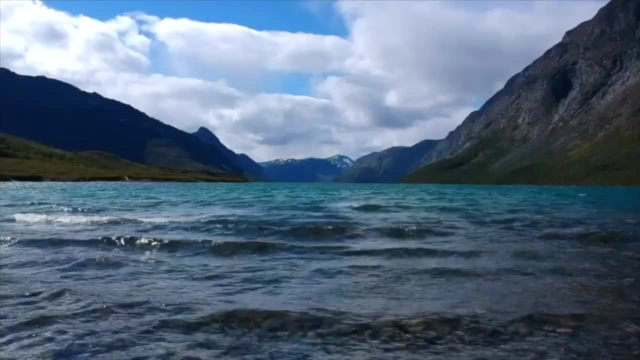 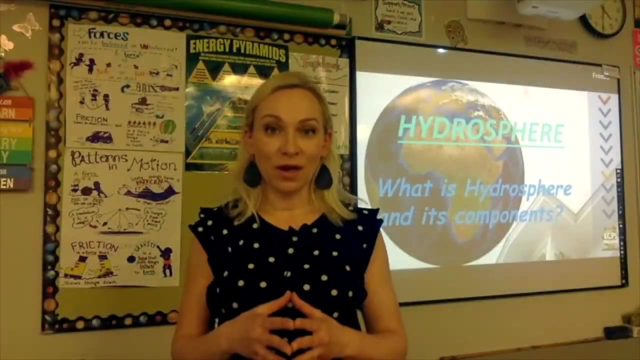 that have to do with the water, like hydrate or fire hydrant. So hydrosphere is made up of water. ice, rain, oceans, rivers and lakes are all part of the hydrosphere. Think about water you use every day When you pour a glass of water at ice, even when you breathe. 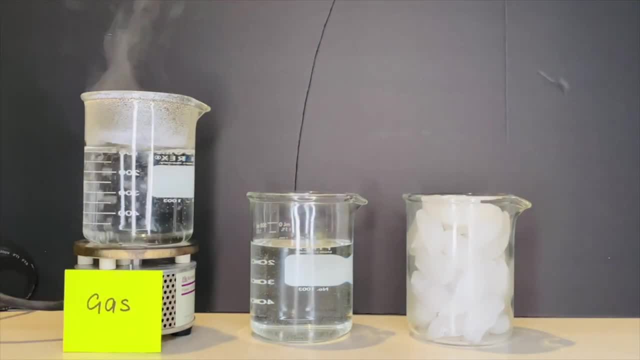 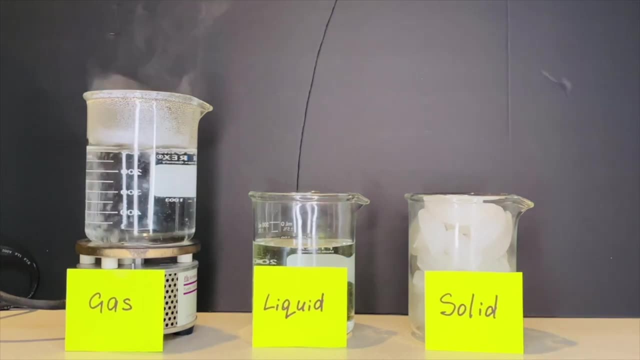 The fact that water exists on the earth as a liquid, solid and gas forms is the one of the unique properties of water. It makes water extremely useful here on earth. One of the reason you can find water on the earth in all three stages is narrow temperature range between. 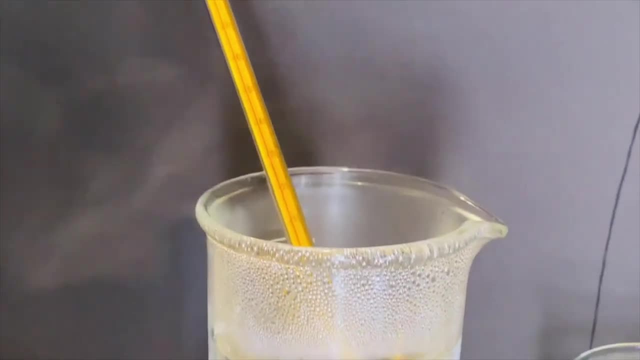 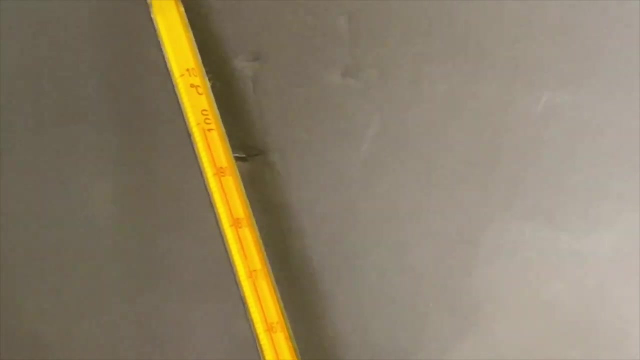 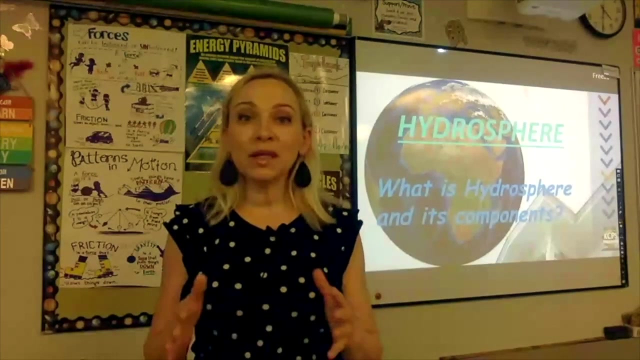 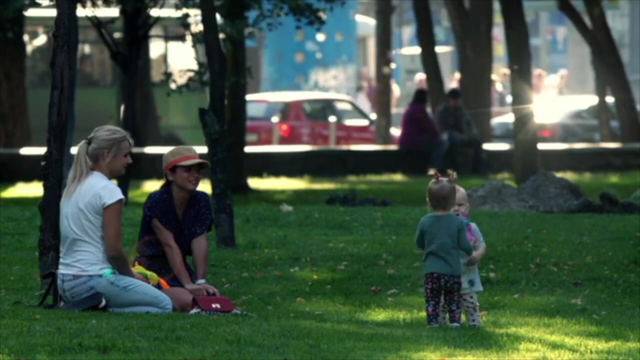 freezing and boiling points. Under standard condition, pure water freezes at zero degrees celsius and boils at 100 degrees celsius. Indeed, without the water, our planet would be completely different from what we know. You already know that we humans can survive without water. Water is all around you. You drink it. 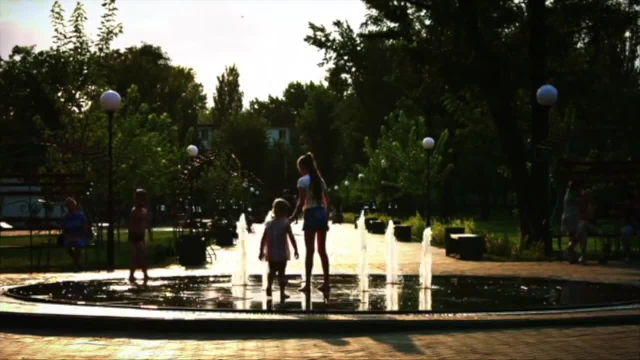 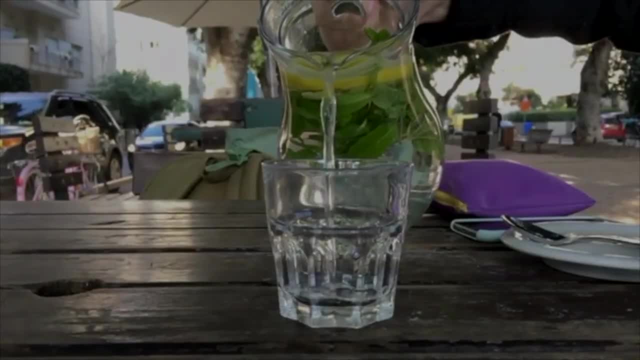 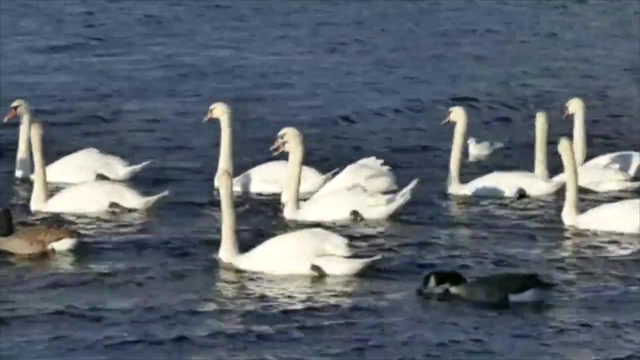 you wash in it, you play in it. Water is through your body. About 70 percent of your body is water. Water not only important to humans, but all life on earth. The ocean, streams, rivers and lakes are full of activity and provide habitats for many organisms. 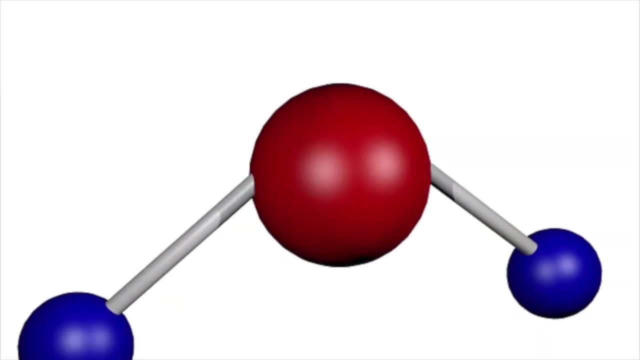 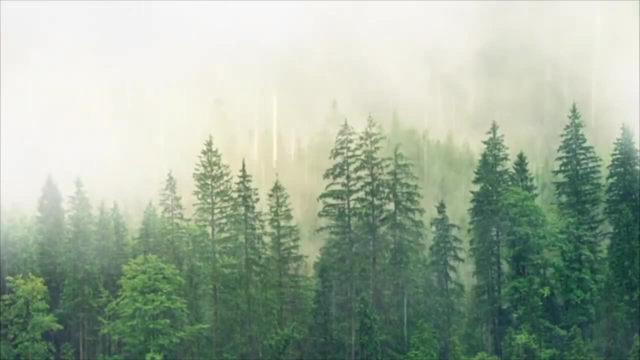 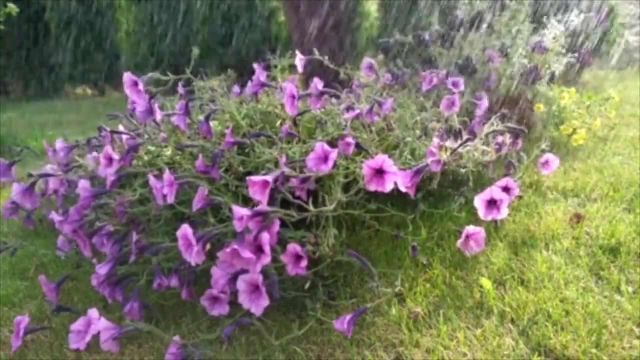 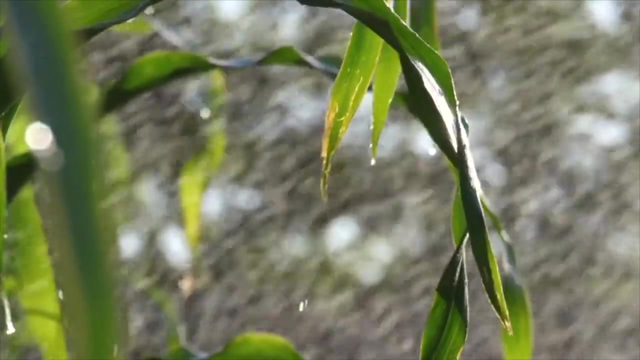 within and around them, Water molecules are attracted to other polar molecules, Together with cohesion. this allows for the capillary action that pulls water upward with narrow tubes inside plant stems. Water moves by this method from the ground to the leaves where the photosynthesis occurs. Animals use water to move in and out of their houses. These are your favorite things to do. This is the first place of water in the world for the population in the United States From the Northern world, you can say that the ocean is the best source of water, for water and it dreams about water. But we also know that the ocean is the best source of water for our plant and we want to able to. 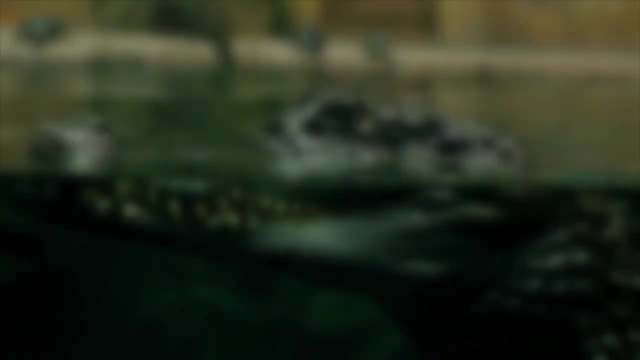 preserve it. In addition to the ocean, we are willing to move water along the risks of this reaction. Water is also an important part of life. You don't need to ever be in contact with any human being to catch anything. use water to move nutrients and waste through their bodies. Humans can survive for weeks without. 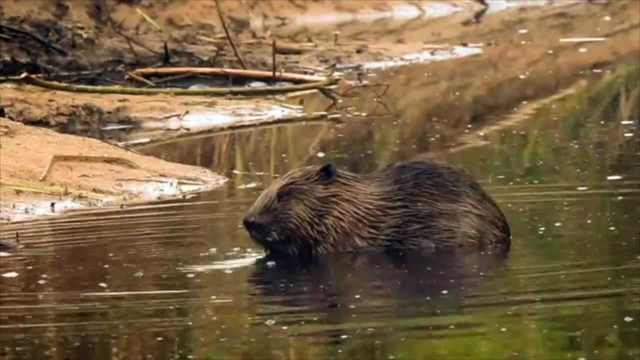 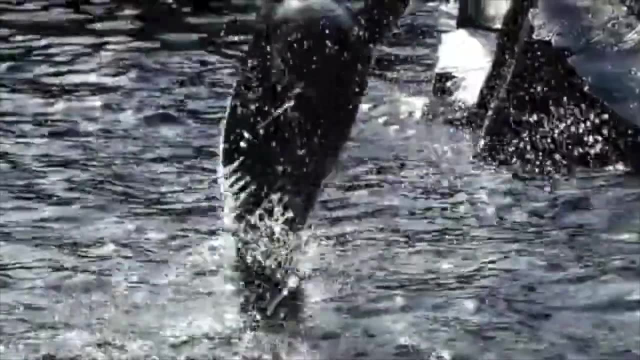 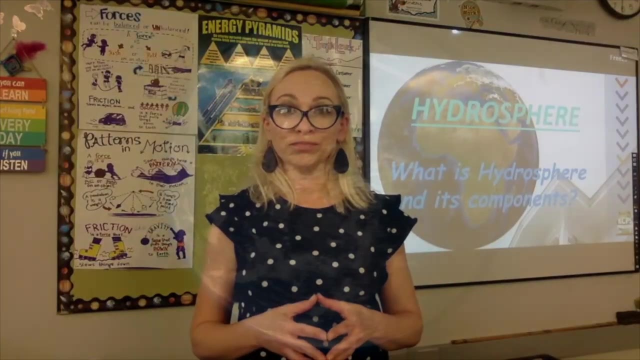 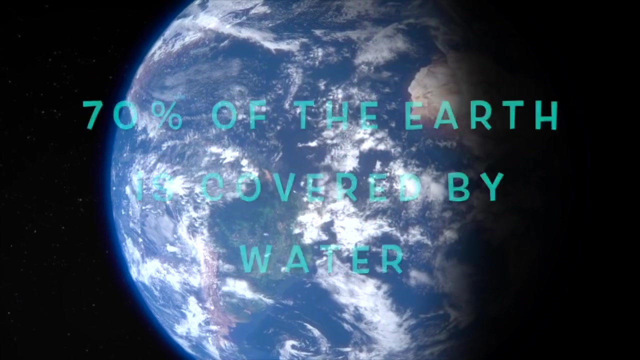 food, but for only a few days without water. How much of the water on the earth is actually a fresh water? Let's find out. Okay, let's talk about where can you find water on earth. Many people call earth the water planet. 70% of the earth is covered by the water. 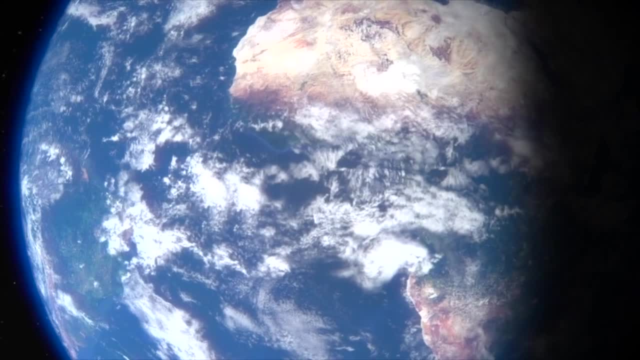 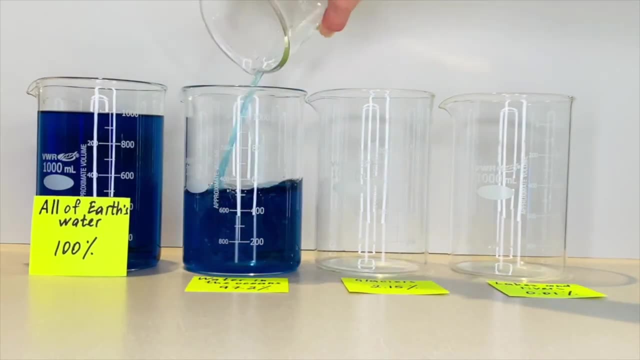 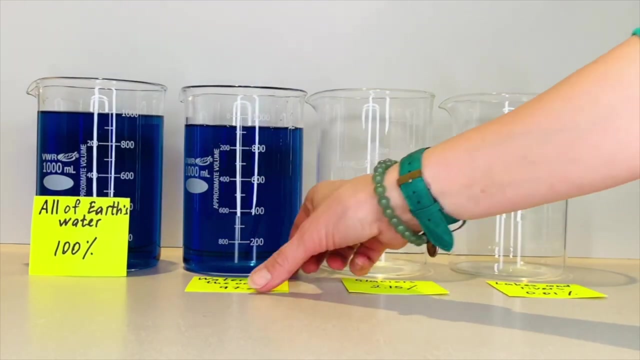 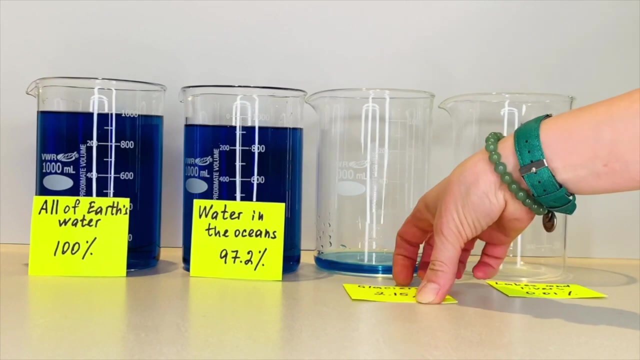 and only small portion is available for human to use. Of the all total water supply, 97% is located in the oceans. This is salt water, so we have just 3% for fresh water left. 3 quarter of that fresh water is frozen in glaciers And less than 1% of the earth's. 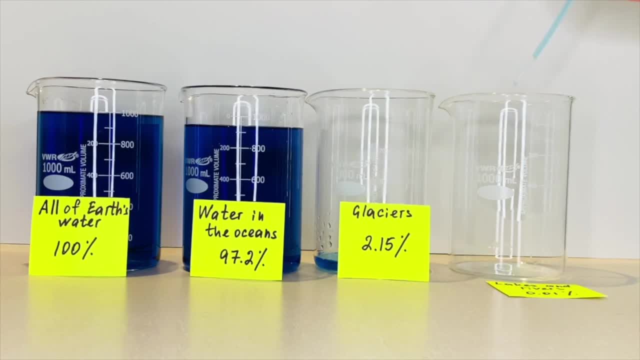 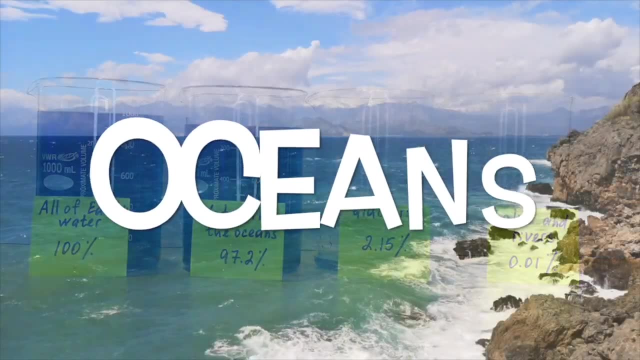 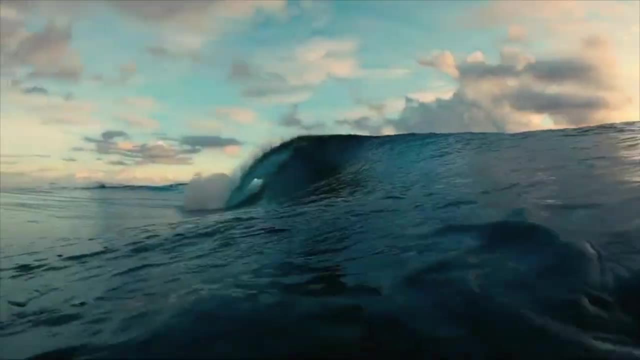 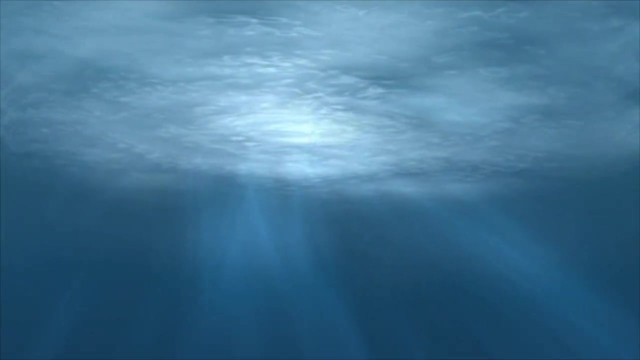 total water supply available for human use, and much of it lies underneath earth's surface. Next we begin our examination of earth's water reservoirs And we start with the earth's oceans. Ocean water is plentiful on the earth, but it is salty and not good for human use. 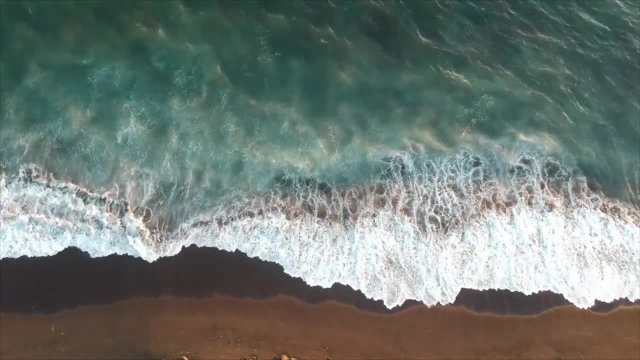 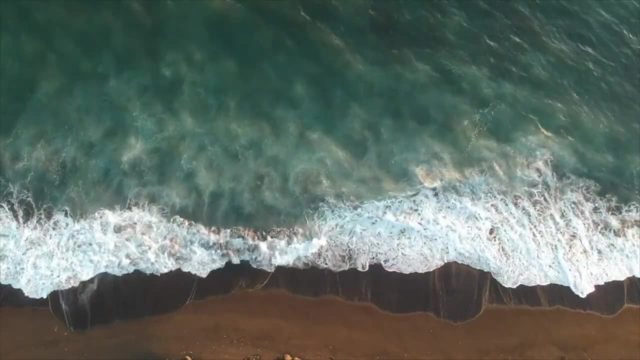 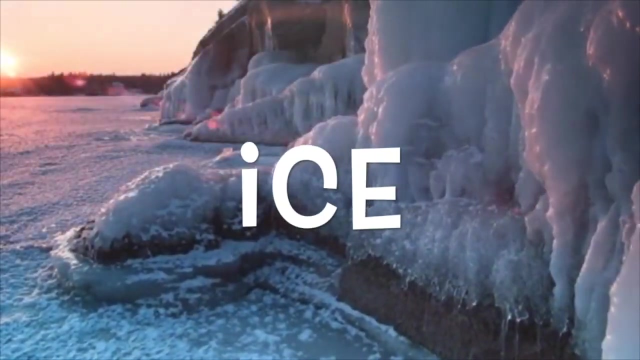 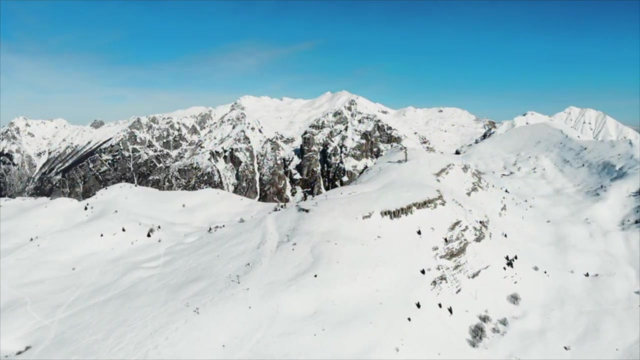 You would have to remove the salt if you wanted to use ocean water for drinking, bathing or irrigating crops. Unfortunately, removing salt from ocean water usually isn't practical. Glaciers are common on the earth's polar regions. for example, large areas of greenland and antarctica are covered. 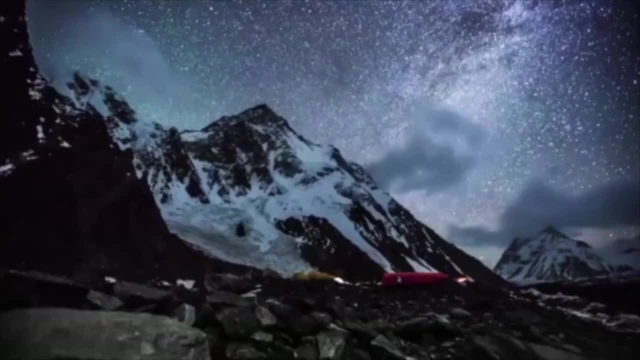 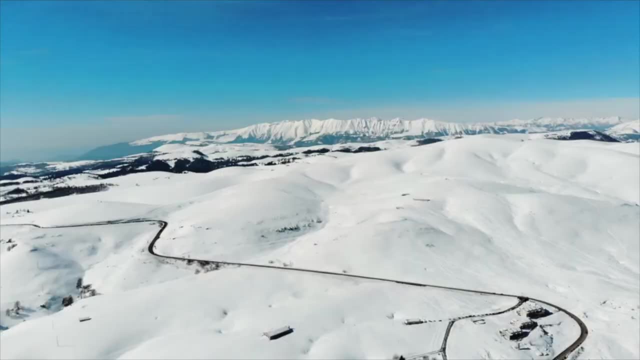 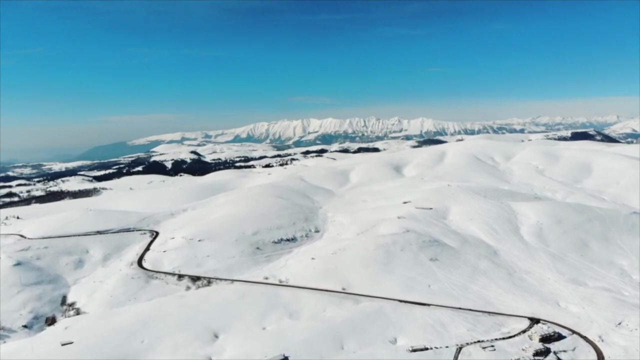 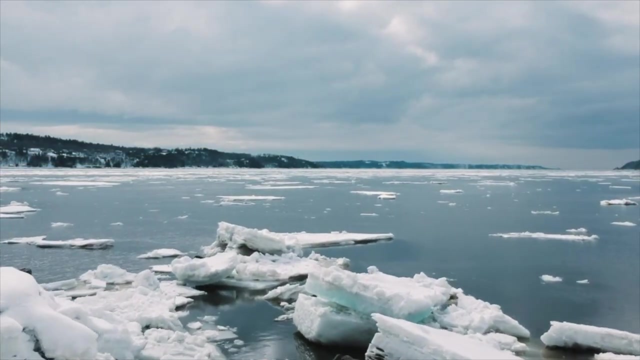 by the ice. these ice sheets look up a large percentage of earth's fresh water. ice accounts for just more than two percent of the total fresh water on the earth, but that is 77 of the planet's fresh water supply. it was proposition of using ships to tow large pieces of polar ice to places. 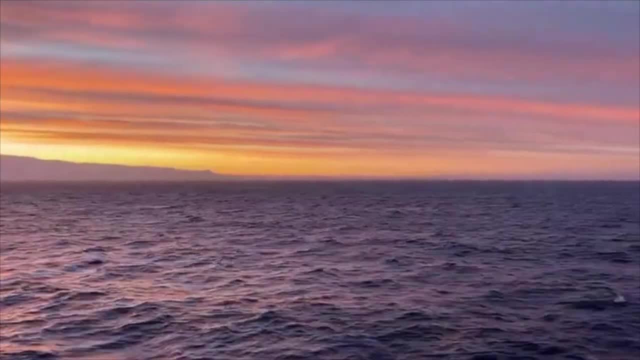 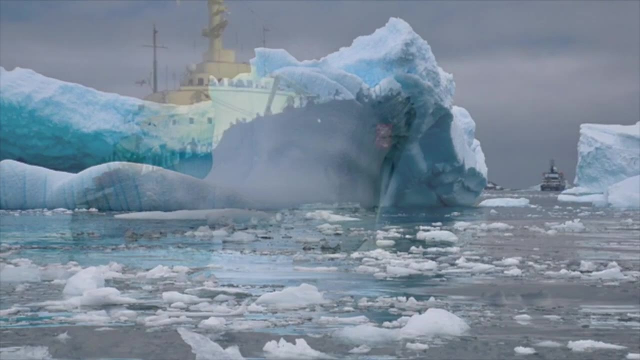 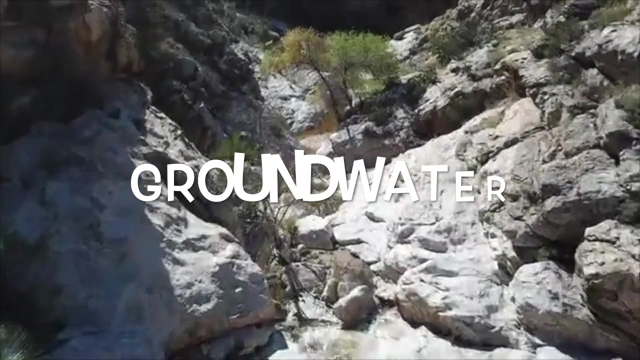 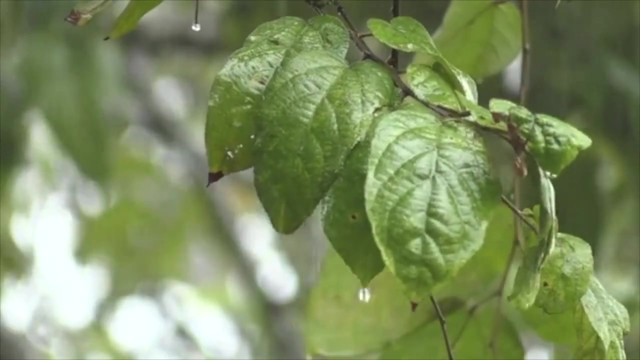 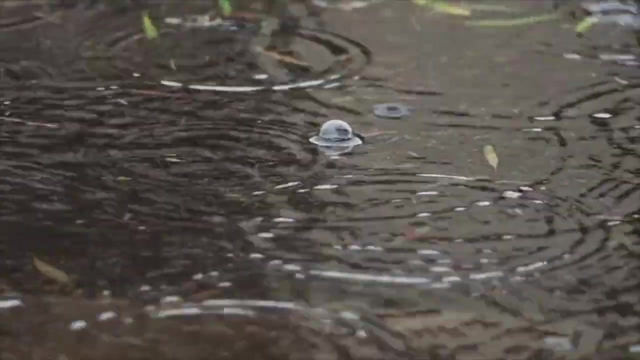 that need a fresh water. it is an expensive proposition and just imagine danger if i should breaks up in commercial shipping lines. our next, a water reservoir. we're going to talk about, um, underground water. you might have wonder what happened to rain after it's false. um, if you leave a bucket outside in a rainstorm, it can be a full quickly with water. 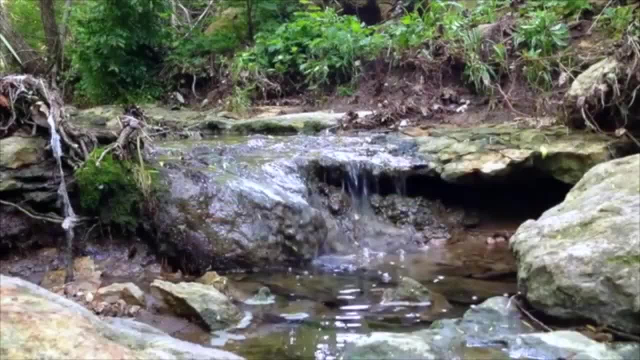 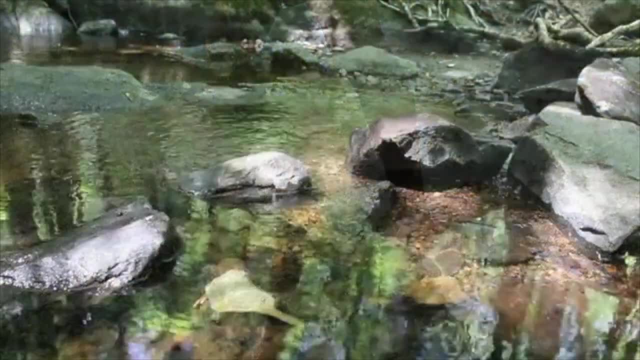 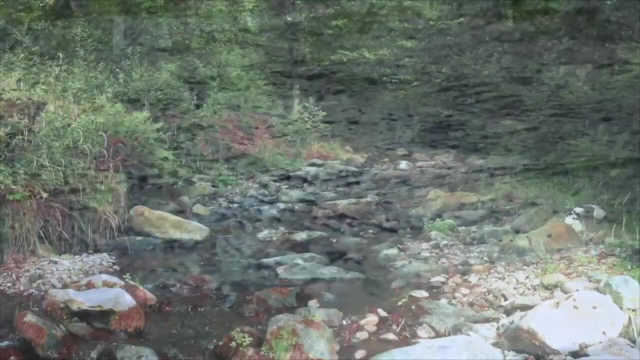 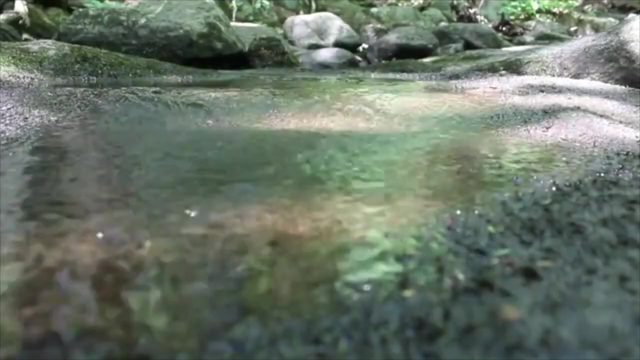 where does the water that lands the ground? where does it go? some of it runs off and flows into streams, and some evaporates a large amount of socks into the ground. water that is held under the ground in the layers of rock and sediment is called ground water, the part of the groundwater that is held within. 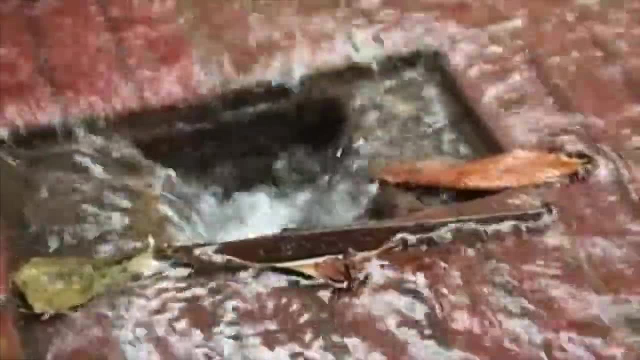 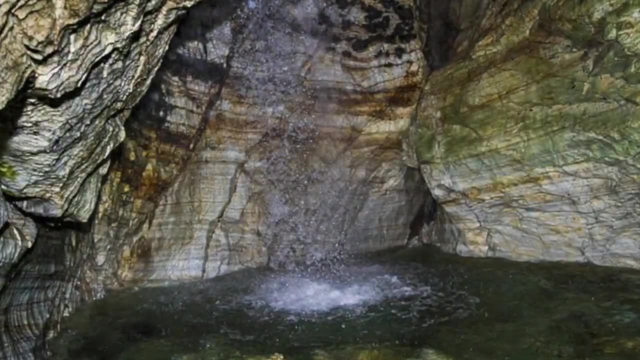 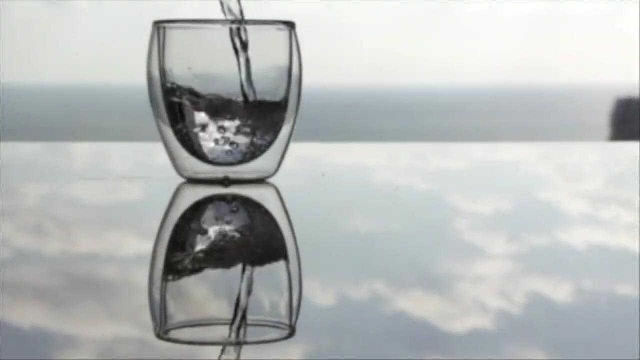 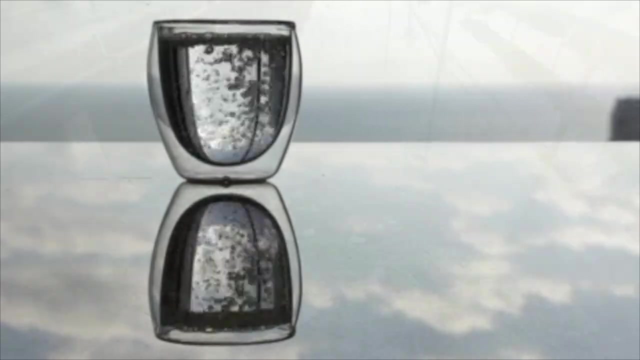 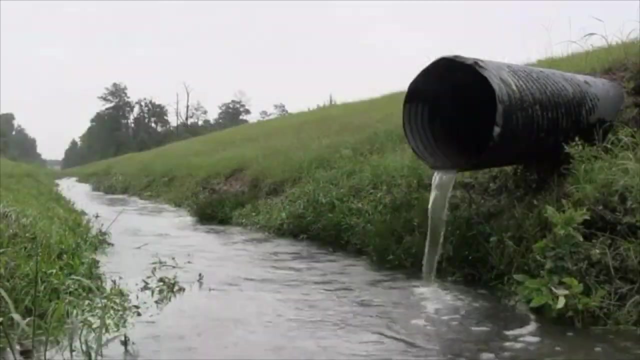 an openings in the soil is called soil water. it keeps plants and crops alive. groundwater also includes underground streams. people in houses that get their water from the ground, so the ground water, water from wells, are a drinking groundwater. the water is purified as it is slowly permits through the layers of sediment and rocks. however, it's a if. 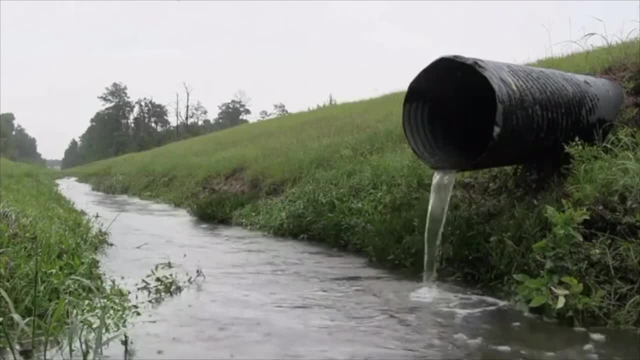 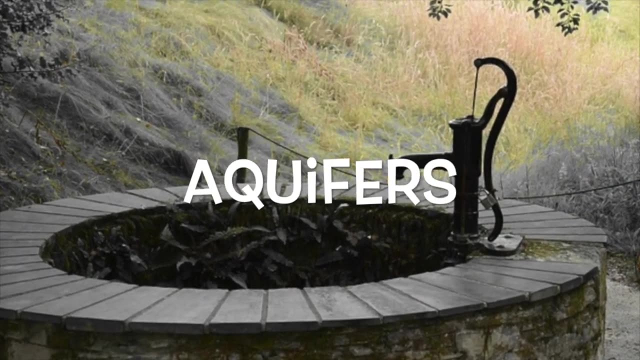 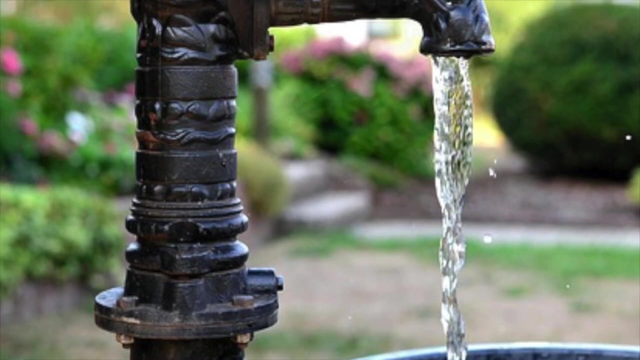 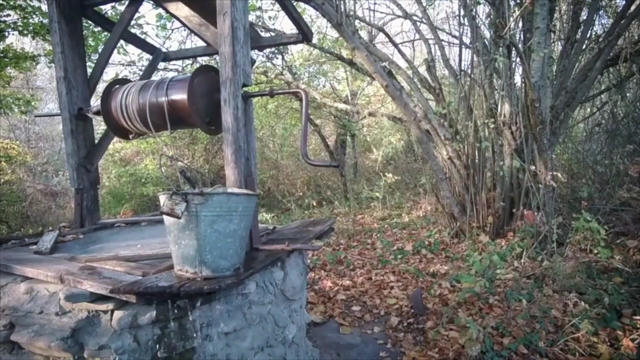 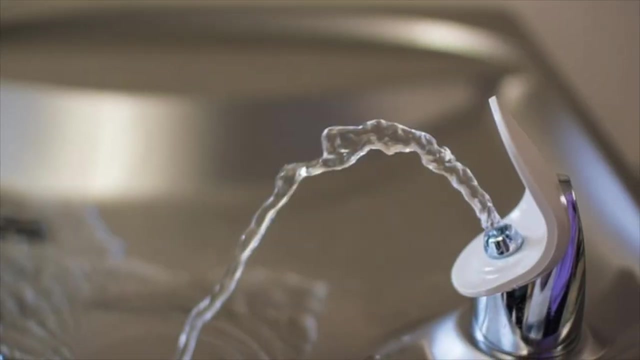 groundwater becomes polluted, it can be very difficult to clean it up, and we are moving on to aqua fears. and aqua fear is a layer of rock or sediment that has enough well-connected openings to allow groundwater to flow through it. water collects in open space between a rock particles. this water flows through 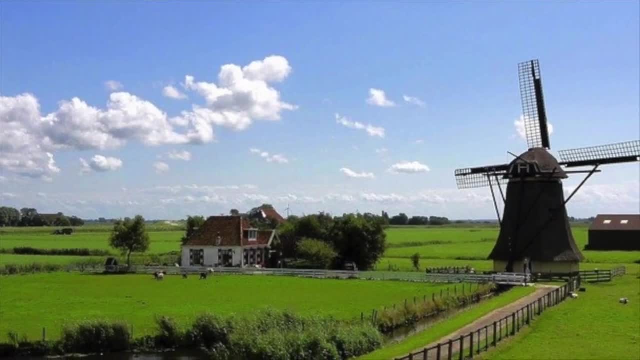 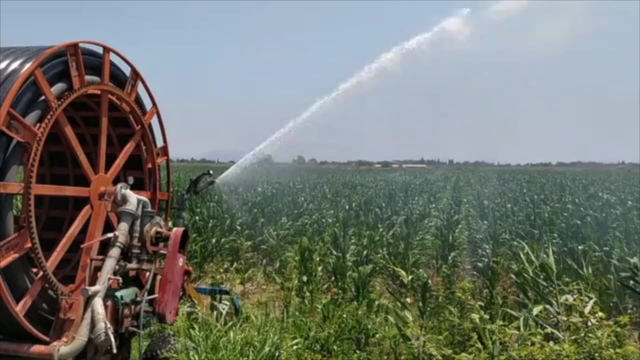 slowly from one open space to another at the rate of a few meters per second, and then it flows through the open space to another at the rate of a few meters per second, and then it flows through the open space to another at the rate of a few meters per hour. that's how slow it slowly it moves, sometimes aqua fires. 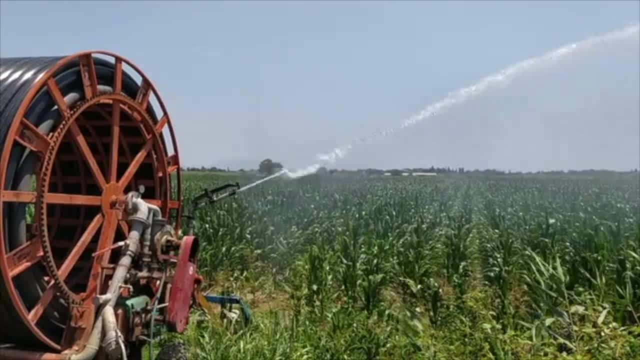 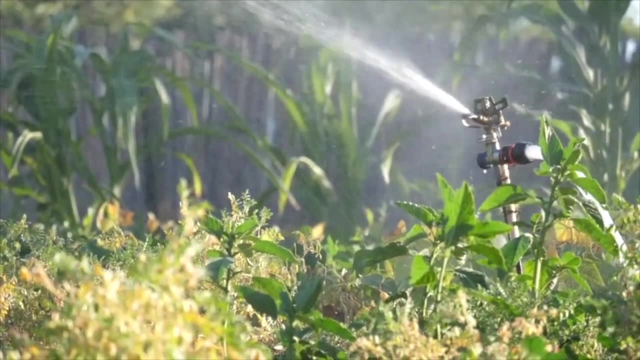 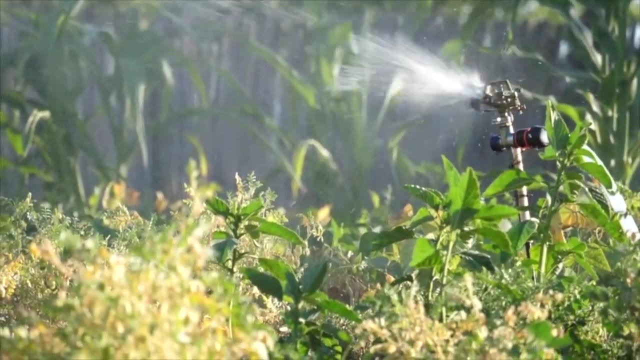 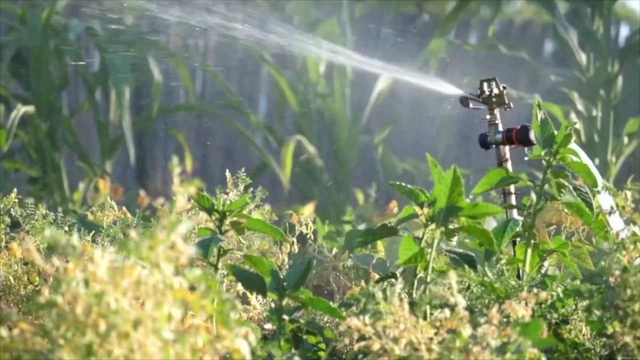 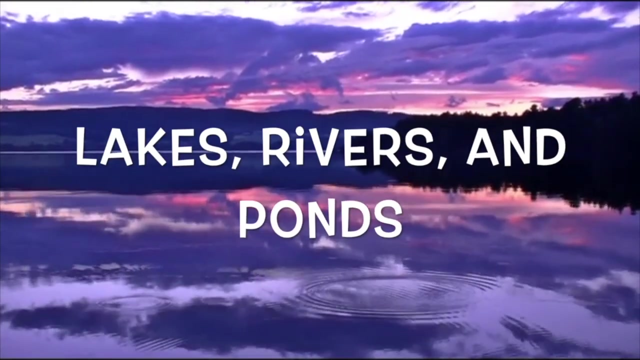 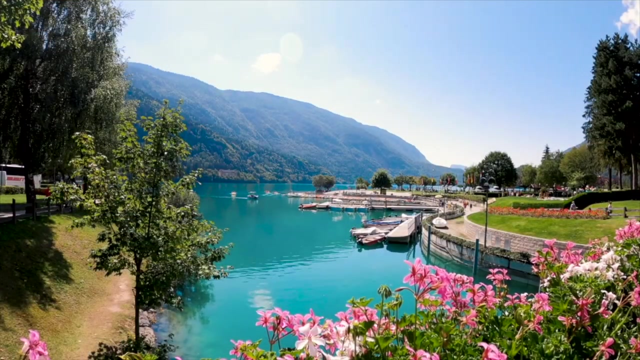 are used to supply water to our towns and farms. the water is pumped to Earth's surface through a well, sometimes Earth's surface deep below the level where the ground water would be. this is where natural, natural lakes and rivers are located. you already have learned about groundwater. the water at the Earth's surface is called surface. 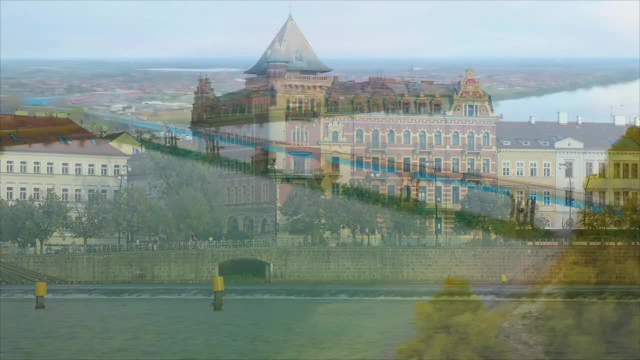 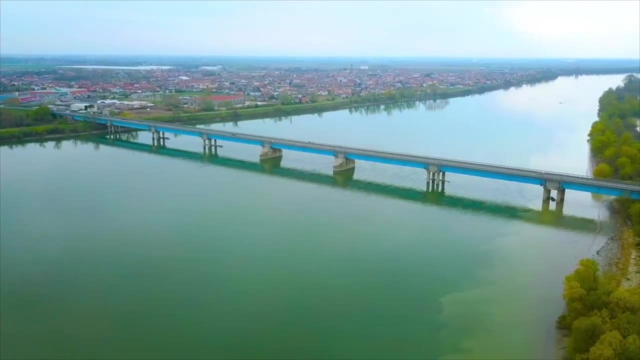 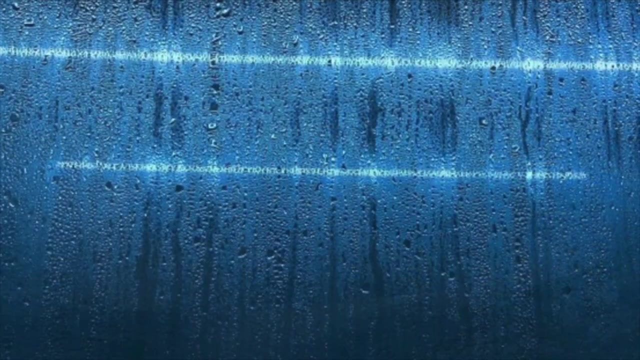 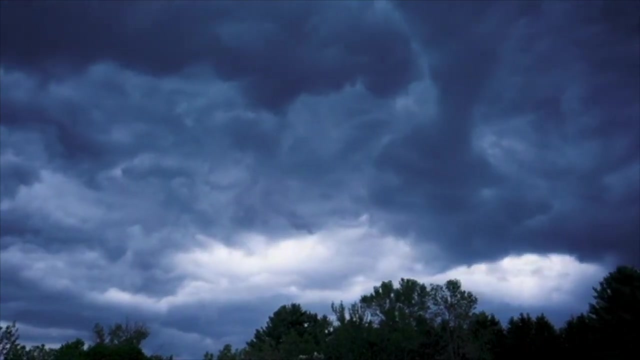 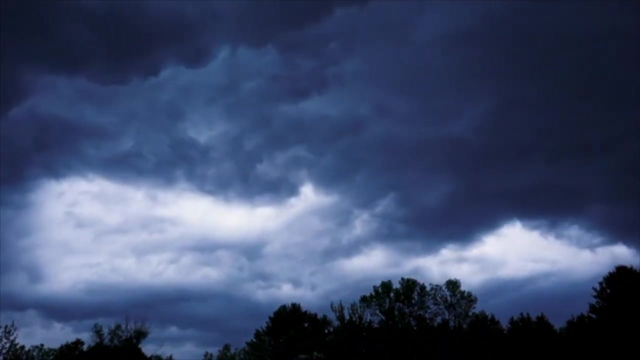 water. it is found in streams, rivers, ponds, lakes and reservoirs. this is water you can easily see and use, and next place where you can find the water is an atmosphere. water vapor in Earth's atmosphere has many important roles. for example, clouds need to be formed, since water vapor is a source of precipitation we will be talking about 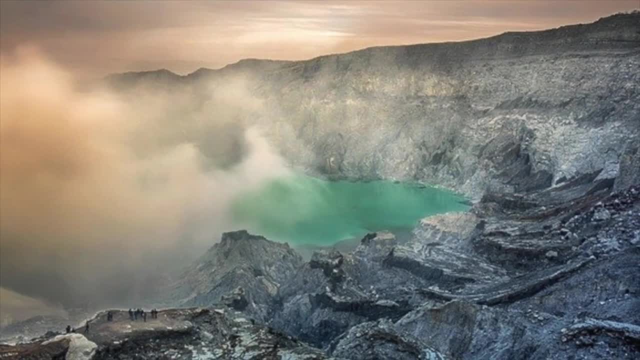 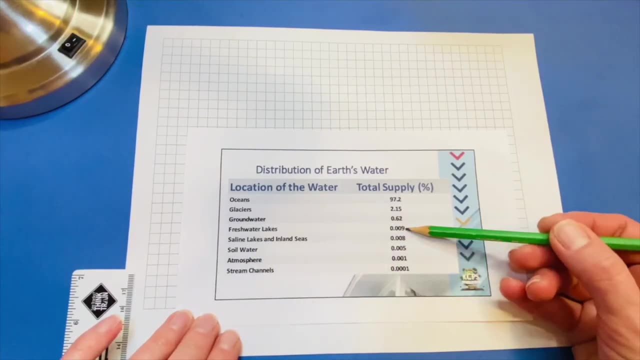 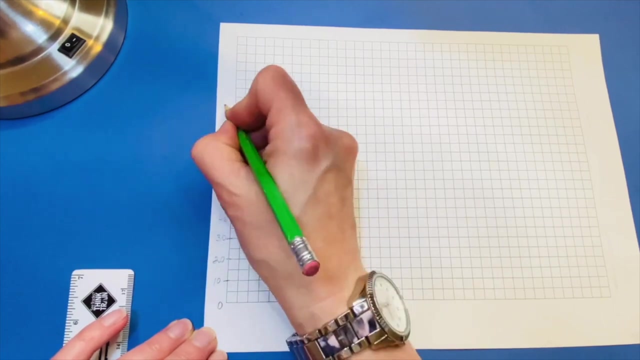 interaction between atmosphere and hydrosphere more in our next video. we will be talking about interaction between atmosphere hydrosphere more in our next video. but right now let's go ahead and move on to our graph. so we're going to create very quickly a graph about amount and percentage of salt water and fresh water. 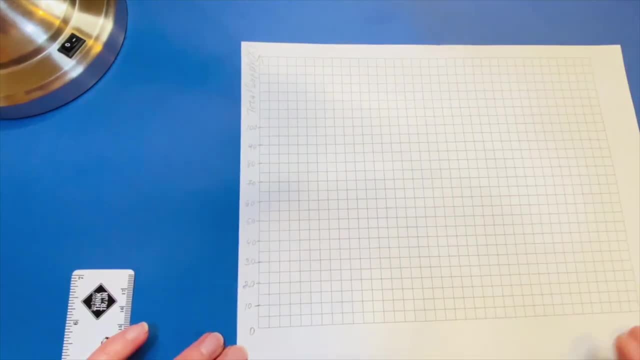 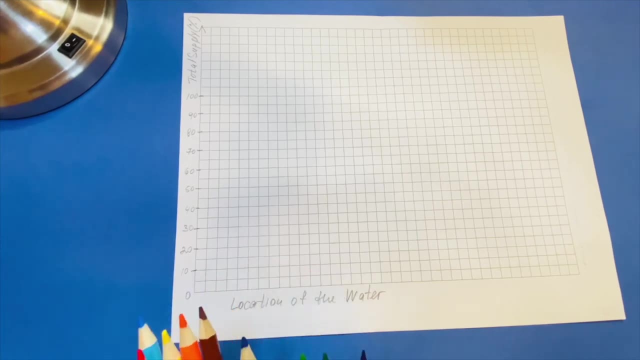 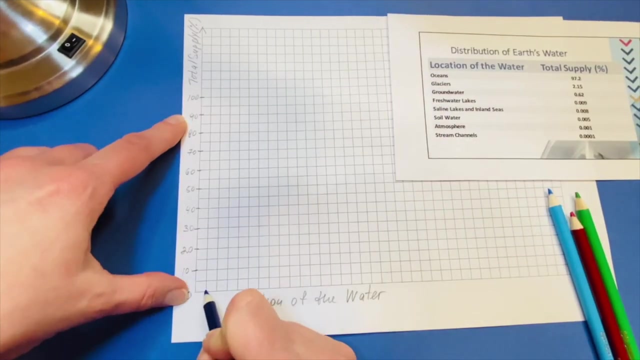 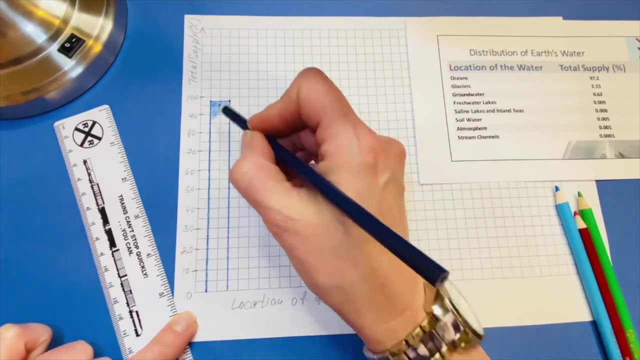 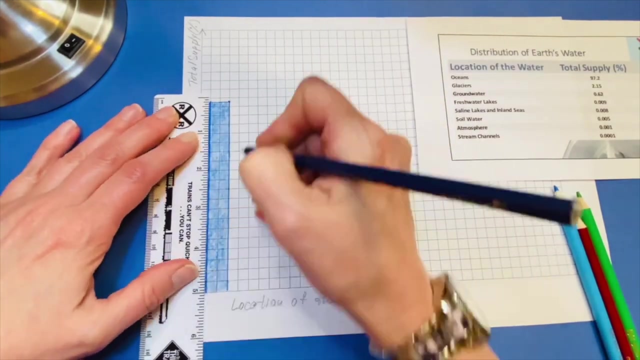 in various reservoirs on our planet. for, based on our data, we're going to use a bar graph to represent distribution of Earth's water on our planet. so we're going to take just the four numbers: oceans, glaciers, groundwater and freshwater lakes- and on y-axis I'm going to put a total supply. 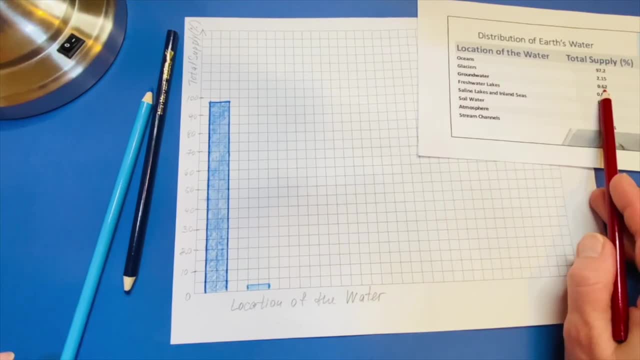 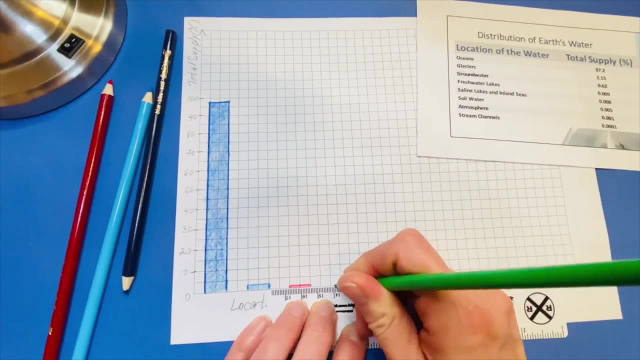 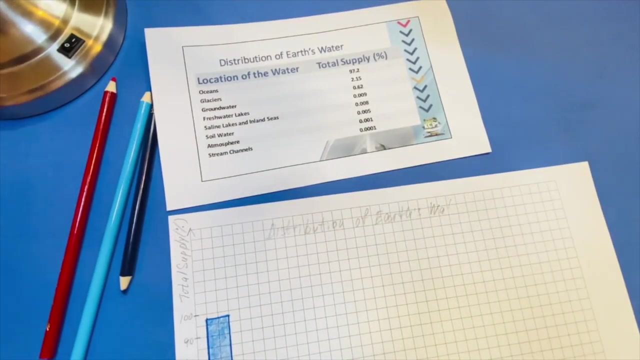 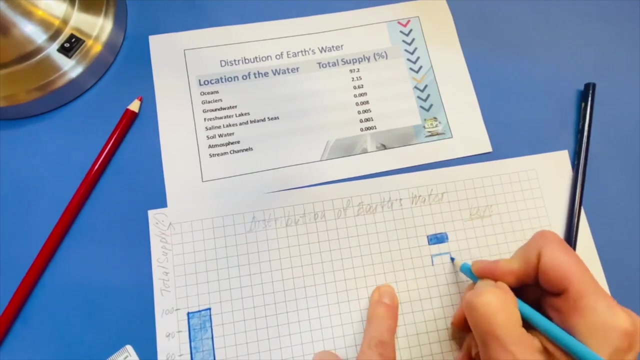 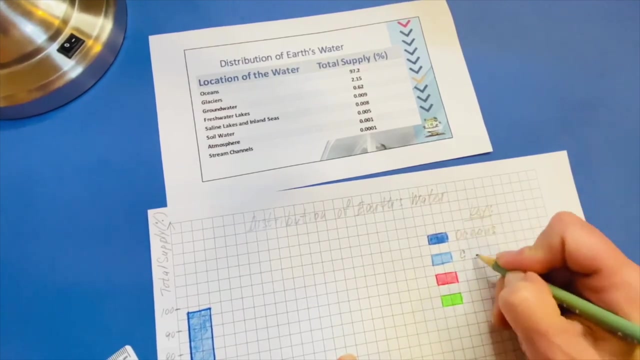 of the water in a percentage, and on x-axis it's going to be a local location of the water, and I also will include the key which will identify which color is: oceans, glaciers, groundwater and freshwater lakes. and, of course, please, please, don't forget your labels on y-axis and x-axis and at the title for